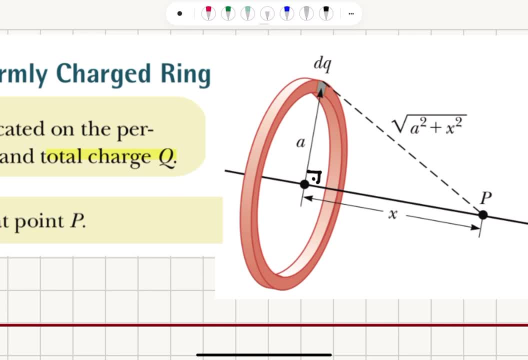 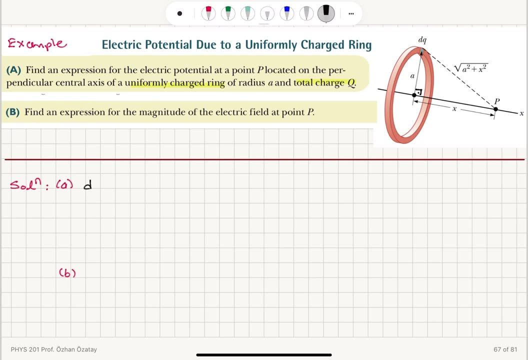 so that's the hypothesis. So the contribution to the potential due to this charge element will be dVp, that is, k, dQ over square root, A square plus X square. So we can write: dVp is k Coulomb's constant, dQ, A square plus X square square root. Then the total potential at 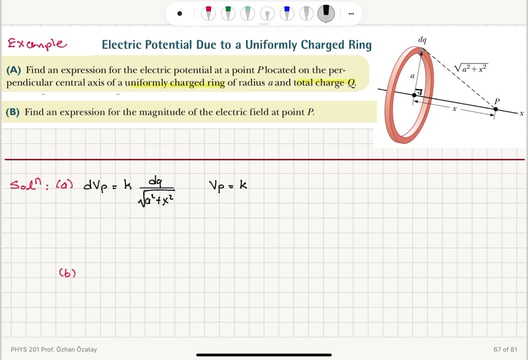 point P will have the sum of the conditions. So again, just to prove these two things, I'll just say we can do the same thing again. When we have the same data, the difference between current emission, current emission and the time- we have the same set of conditions. So I will use c Coulomb's constant dQ, DQ, A square. 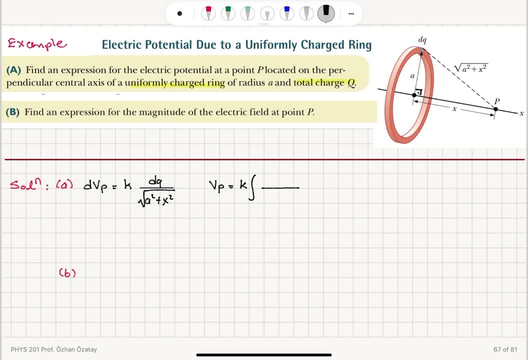 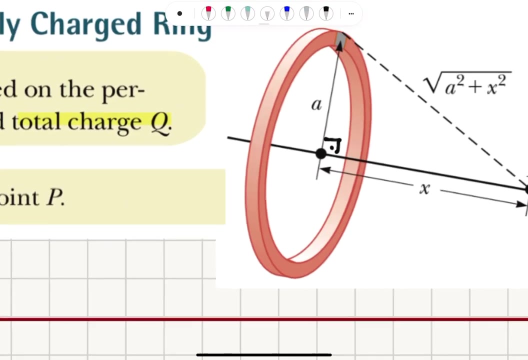 plus X square square root. A square plus X square dQ. A square plus X square square root of dQ. A square plus X square square root. Then we end up with these conditions. We can see that for each charge element that I pick on this ring, here, here, here, here. 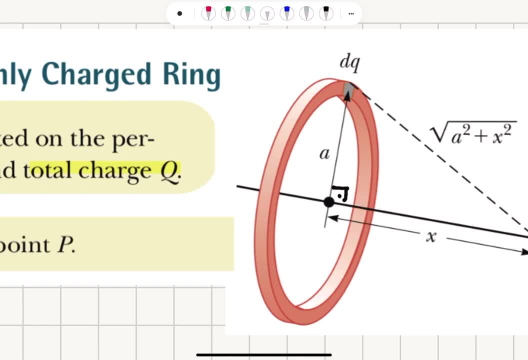 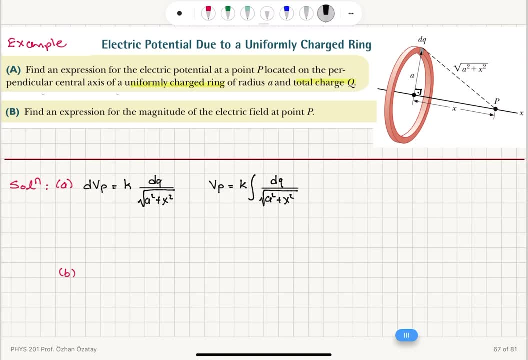 it doesn't matter, since this is the perpendicular central axis, I will have the same distance square, a square plus x square. so that will come out of the integral. so this will be k divided by square root of a square plus x square, and then i have the integral of dq. well, if i integrate over the whole ring, i will obtain: 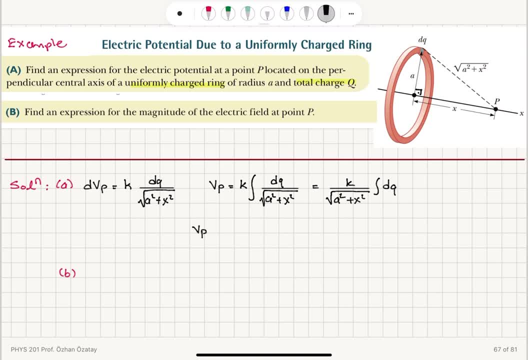 the total charge. therefore, the potential at point p can be written as coulomb's constant k. total charge q divided by a square plus x square square root. so this will be the total potential at point p due to the continuous charge distribution. now, as for the electric field at point p, you can see that when i pick a charge element. 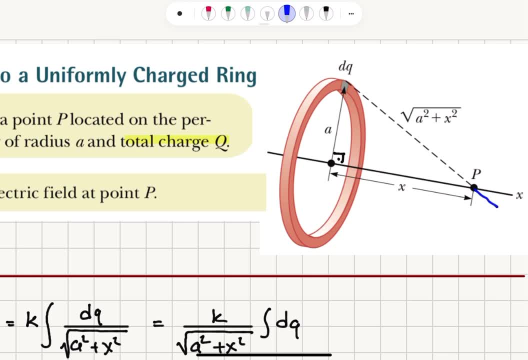 dq, the electric field due to that charge element will be in this direction. if i pick another charge element, dq, which is symmetric with respect to the central axis, then i will find that this charge element will have exactly the same electric field as the charge element of the electric field. so that's why i have the electric field. 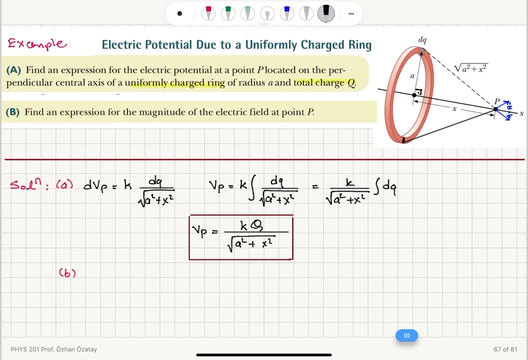 being applied and you can see that the y components will would cancel each other. okay, so therefore we can say that the y component of the electric field at point p is zero due to symmetry. okay, on the other hand, knowing the potential gradient of the potential, so i can find the x component of the electric field at point b. 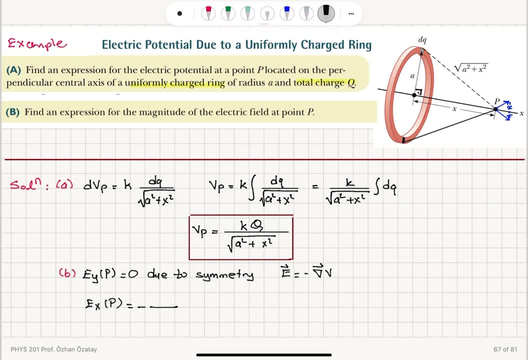 as minus derivative of the potential with respect to x dv dx. this is minus kq, the derivative, with respect to x d dx, of a square plus x square to the power minus 1 over 2, and this will give me minus kq multiplied with minus 1 over 2. 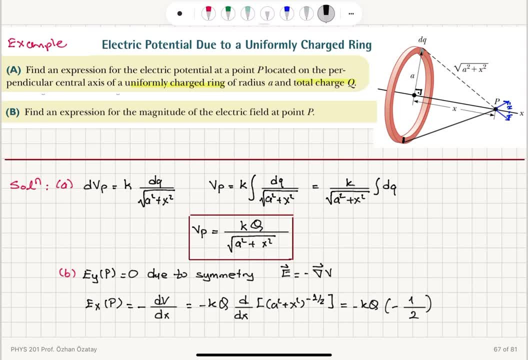 minus 1 over 2, and then i have the derivative of inside, which is 2x. then i have minus 3 over 2 power. so this will become a square plus x square to the power 3 over 2.. now you can see that the twos will cancel and the minus signs will cancel. 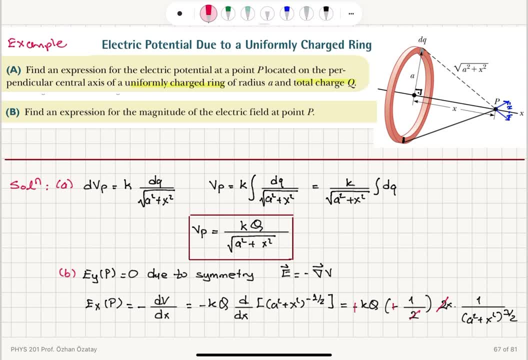 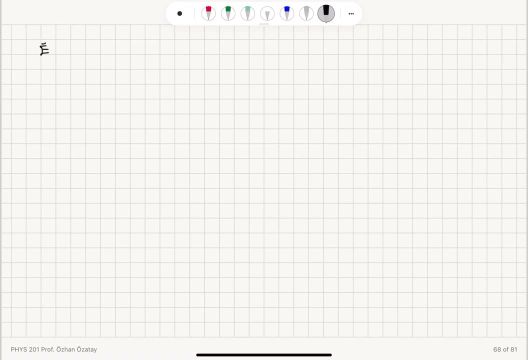 i will be left with a plus and this will give me the x component of the electric field. but there is only x component because the y components cancel, as i have shown here. so we can write the electric field at point p as kq, x divided by a square plus x square to the power 3 over 2 in i hat direction or x hat direction. 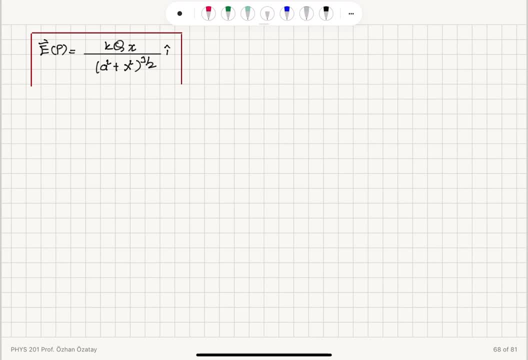 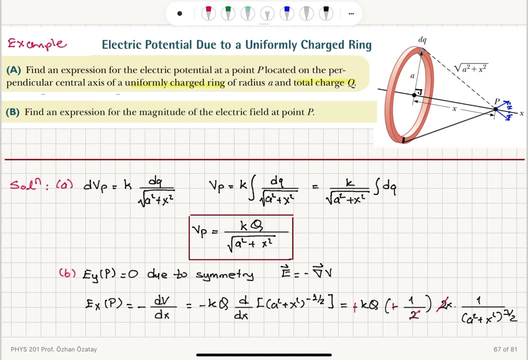 so that will be the total electric field at point p. okay, so in this problem we have considered an example of a continuous charge distribution: the uniformly charged ring. the uniformly charged ring carries a total charge q and has radius a for each charge element that i pick on the ring.